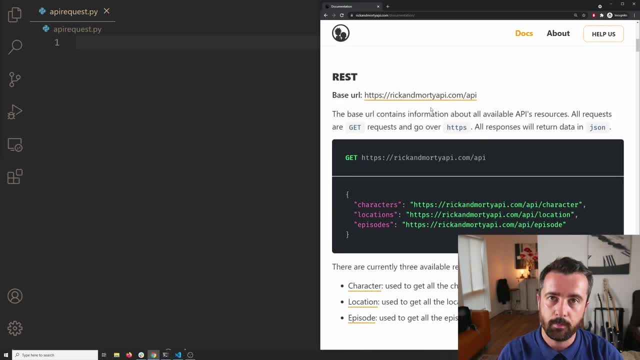 another time. but also it has a good REST API and even better documentation, because the first thing that I would always say when you're trying to work with a specific API is: you need to go through their documentation so you can work out what information is where and how you're going to get it out. 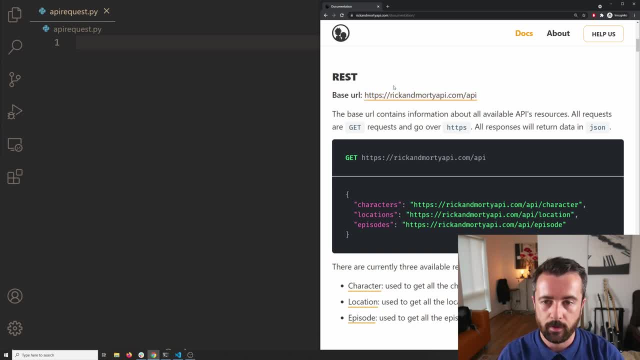 So if we look at this, we can see we have a base URL for our REST API. Now, this is important- We're going to take this as well- and we can see that if you hit this endpoint, you actually get this information back. 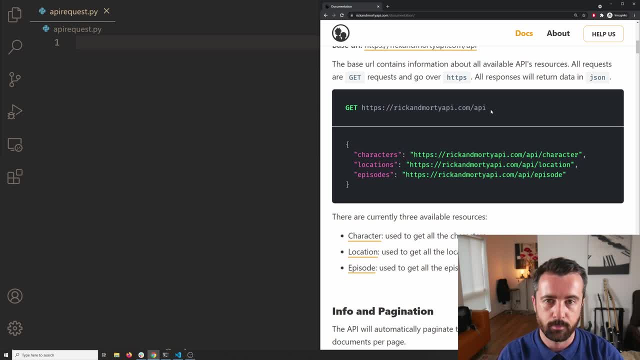 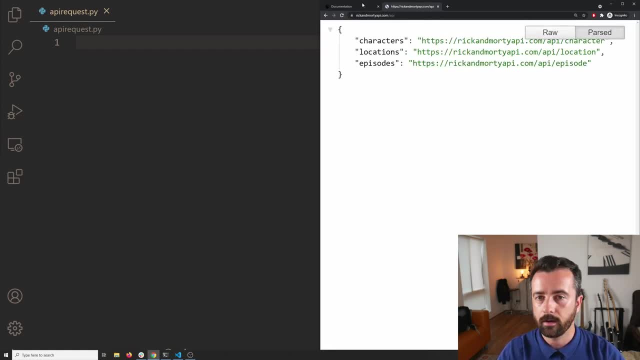 Which tells you that you can query for characters, locations and episodes. What I'm going to do is I'm actually just going to copy this, I'm going to paste it into my browser and we're going to see that we get this information back. here is what we saw right here. 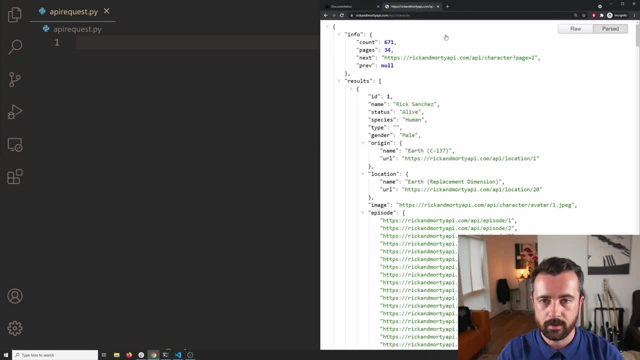 So what we can do is we can actually just interrogate this as if we were working with a website, although we're actually looking at and asking the API for bits of information. So I'm just going to make this bigger right now so we can actually see what the main response looks like. 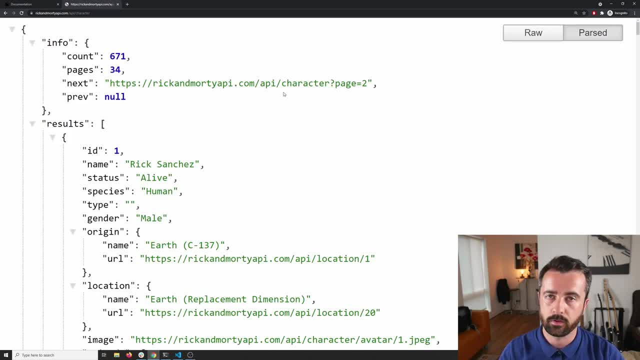 So, before we go ahead and actually look at the REST API, we're going to take a look at the REST API and actually start working with the code. I'm going to run through this response here and explain what all these bits are. now It's really important because when you actually look through the API, it will give you a response and a schema of what. 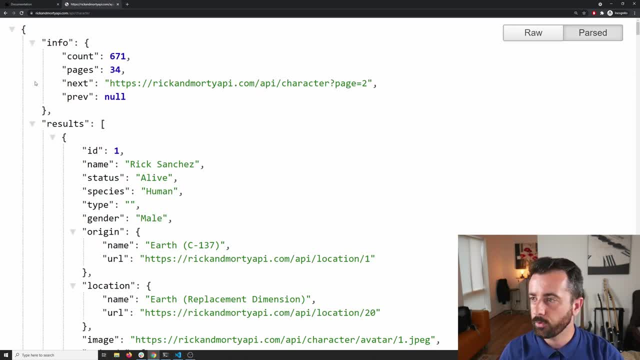 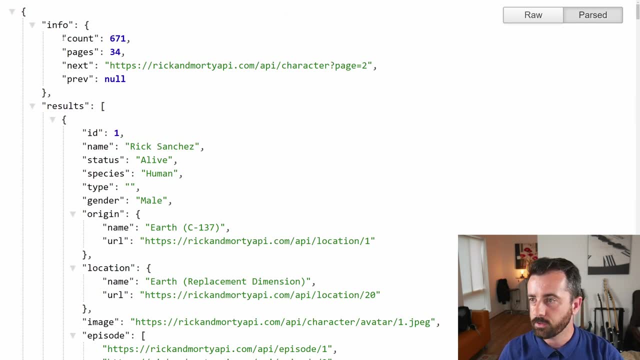 the actual data is coming back. So we can see that we have two main things here. We have the results and this info thing at the top. So the info bit actually tells us how many results there are for the endpoint that we've queried and how many pages. 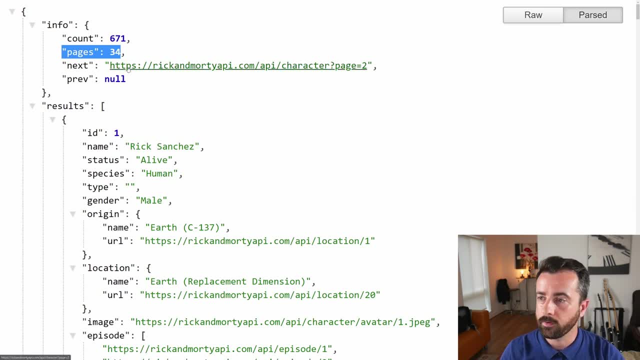 there are. Now. this is going to be really important information as we go forward, and it also gives us the URL to the next page. You don't always get this, but there will be some kind of total number of results and also number of pages, or some do it. 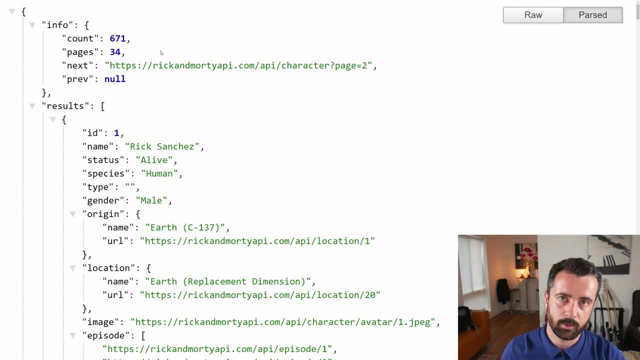 by you do the next load of results. So it would be: the first would be one to 100 and then the second would be 100 onwards, et cetera. But in this case we get a total count and a number of pages, so we can collapse that. 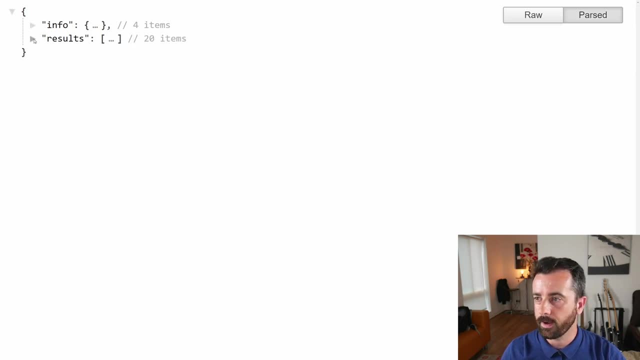 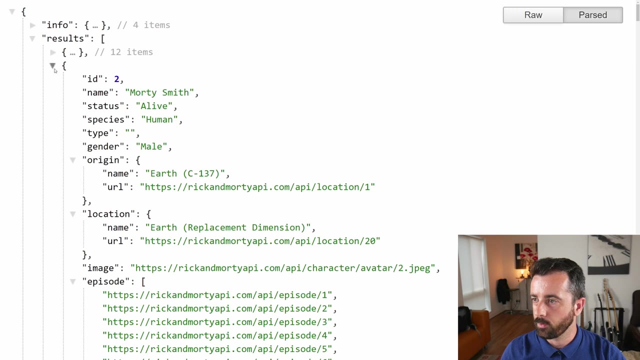 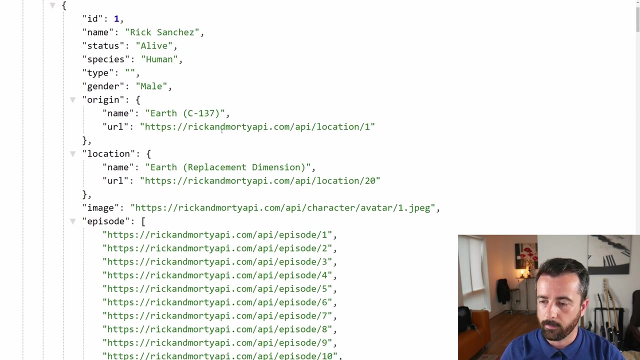 And now we can see that we get a list of results. So if I collapse that, we can see that my browser is telling me there are 20 items and we can see that we have all 20 here and each one has 12 specific bits of information in it and ID name, et cetera, et cetera. 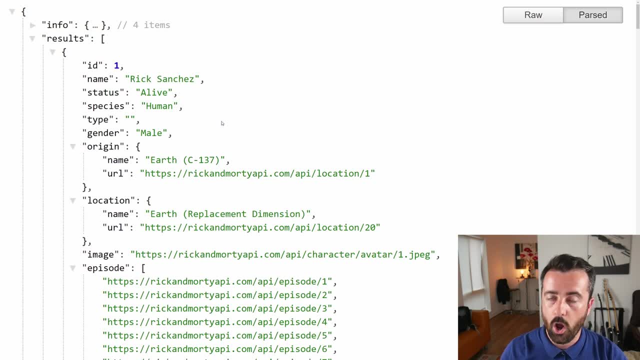 So what I'm going to do is I'm going to say that we want to compile our own list, for whatever reason, of characters from this TV series. we're going to take the name and then maybe the list of episodes, or that might be quite long, but 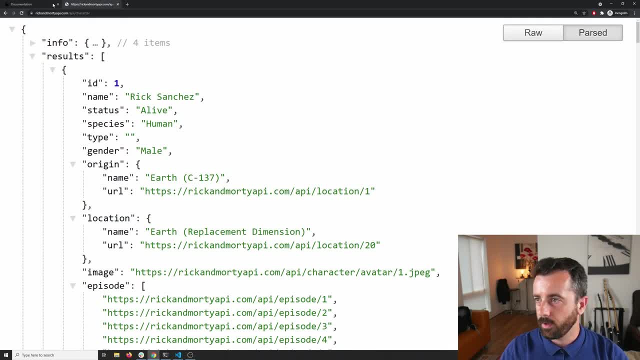 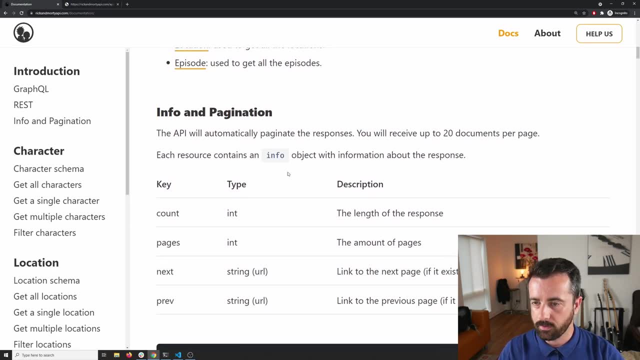 we'll see When we get there. So what we want to do now is going to come out of here and we need to go back to the documentation and we can see that we have what I just explained here. It tells you that the information given, et cetera, et cetera, and then the character end point, which is what we just looked at. 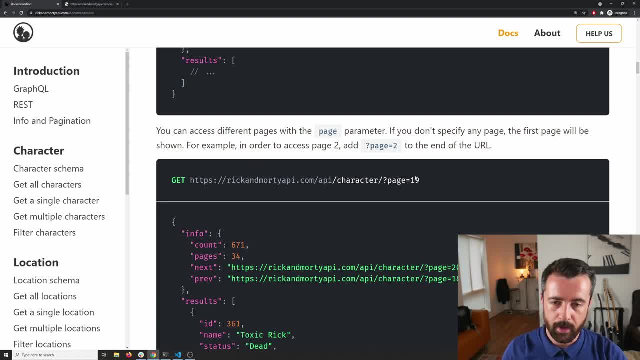 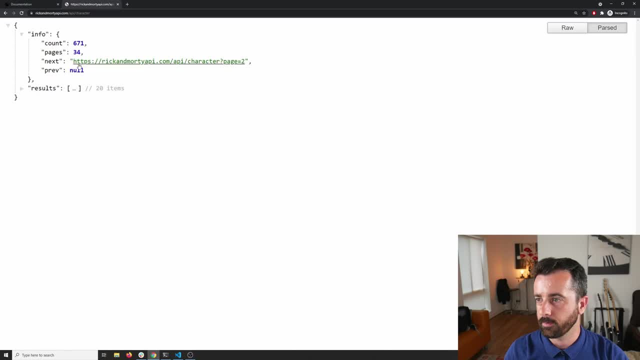 So it says you can access different pages with the page parameters. So that's really important And we saw that in the next link when we looked at the information up here under the info tab you can see it says next page is equal to two. 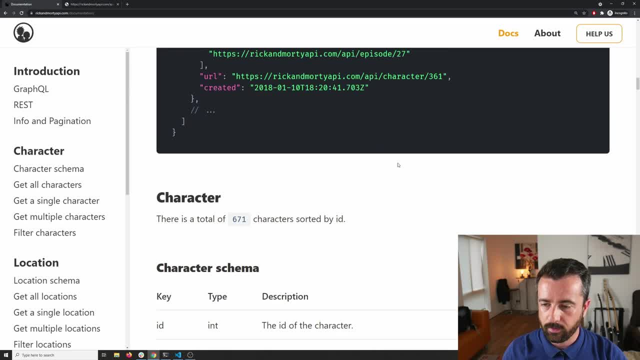 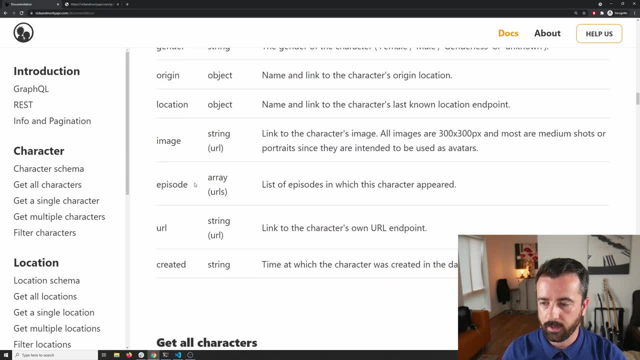 That's a really common way of doing it. Then we have all the information, et cetera, et cetera, And you can actually see the character schema here that I showed you, with all the information you can get out, et cetera, et cetera. 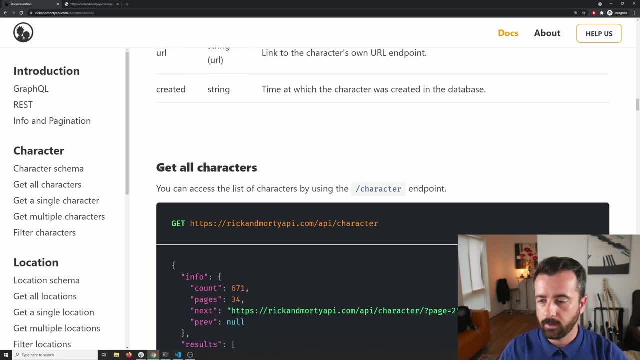 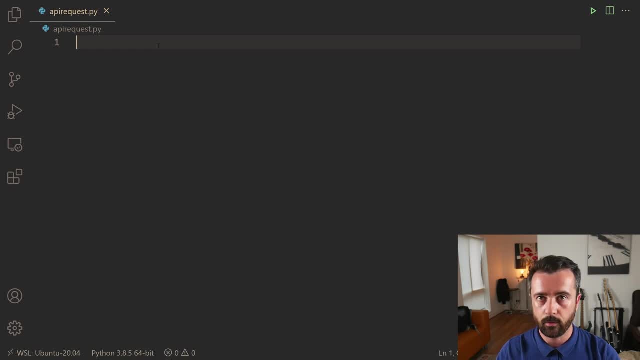 So we're going to do: get all characters. This is what we're going to do, So I'm going to copy this URL here and we're going to go to our code now to make requests to a server using python or anything like that. 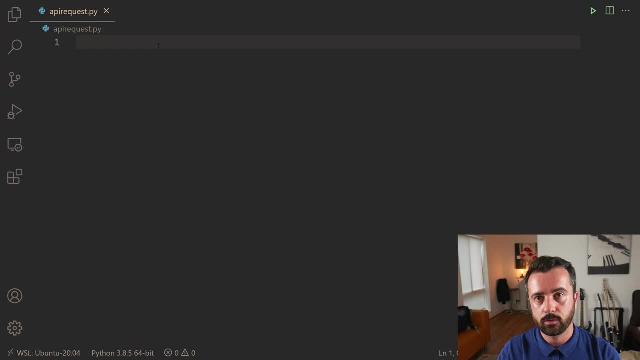 We need to use the request module. If you don't have this installed, you can do pip: install requests. You can google that, You can find it. That is the main one that we're going to use. Even the main python documentation says to use requests. 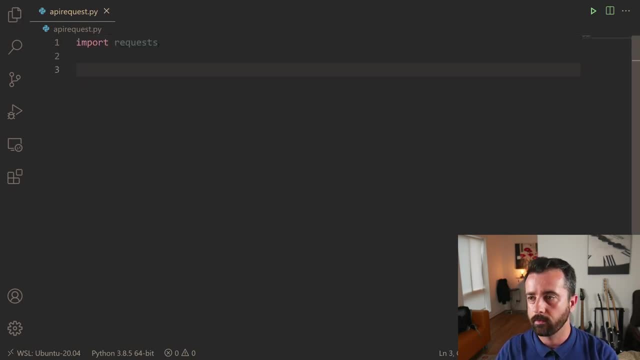 I already have this installed, so I'm just going to import requests up here at the top, like that, And then I'm going to set my base URL to this, But I'm going to remove the character part, because this is the base URL that we're going to use. 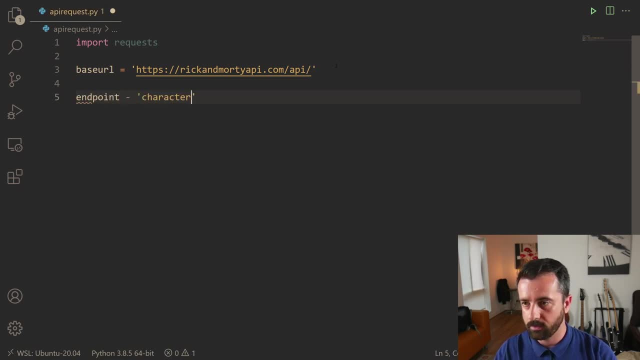 And then I'm just going to say that our endpoint is equal to character. Now, notice that I've left the training slash on our base URL. So now, when we hit, This equals. Sorry there, what I'm going to do with this is I'm going to make a request to this API with us, with our code. 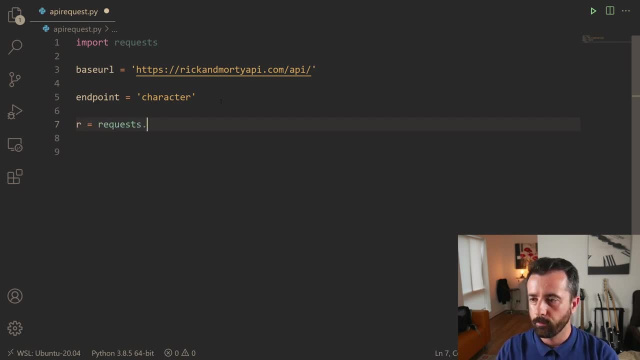 So I'm going to say r is equal to requests and we're making a get request, So we're going to do dot, get. then we're going to say our base URL plus the endpoint. now, because these are both strings, We can just use the plus symbol to concatenate them together, and then I'm going to print out our. now, when I run this, we are going to get back a response of two. 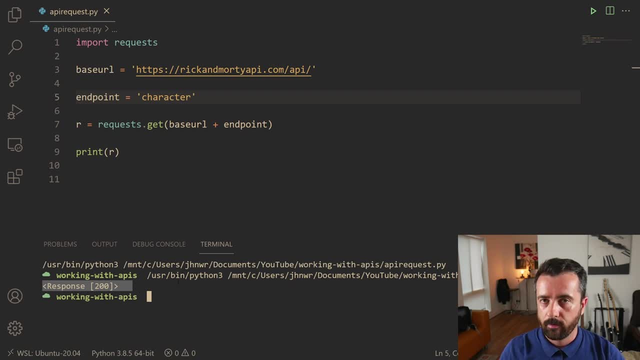 Which is a good response If you're getting something other than that. 400 or 404 is not there. 500 is usually excess denied or something like that. But now we actually want the, not the actual response code. We want the information that's in that response. 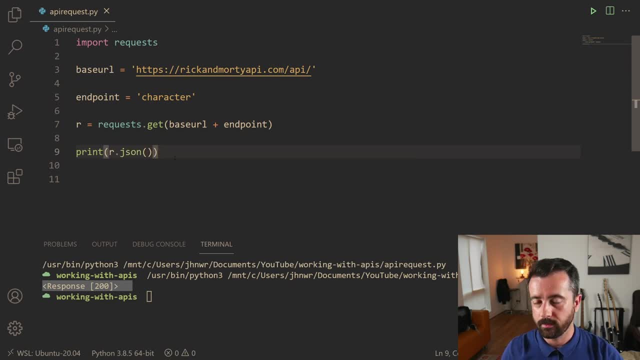 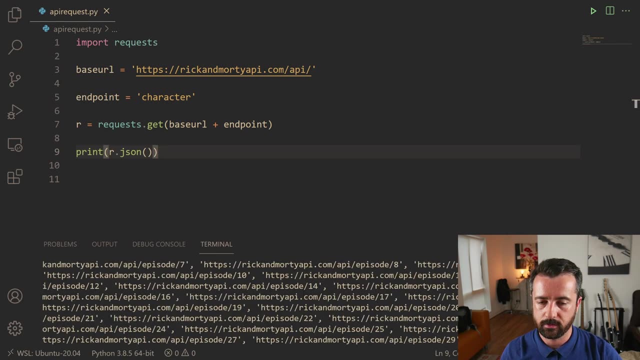 And the easiest way to do that is to r dot jason And this is going to give us the jason response back from the API. So I run that whizzes by on the terminal. We can see we get a load of information back and this is exactly what I showed you in the browser. 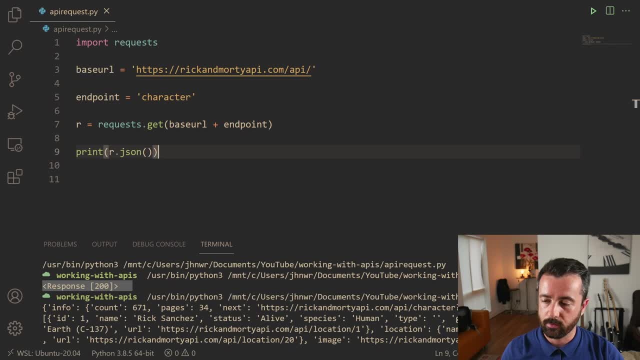 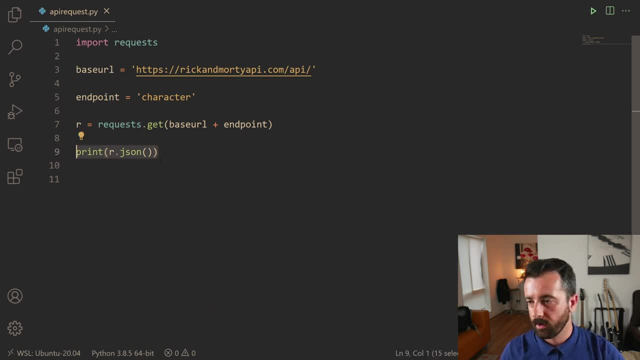 Except Now we can actually do stuff with this response and we can take this information out and we can get the bits that we want. So what I'm going to do is I'm going to say: let's say data is equal to r dot jason, and then I'm going to say print and we're going to say data. 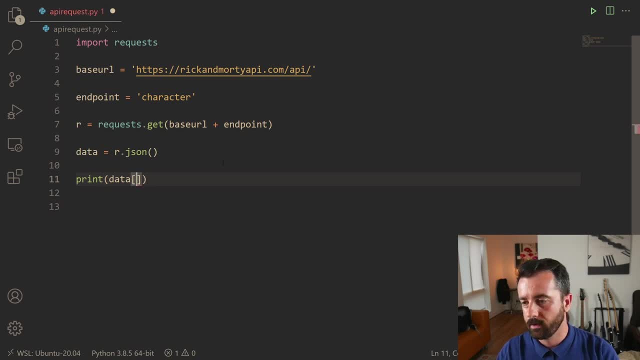 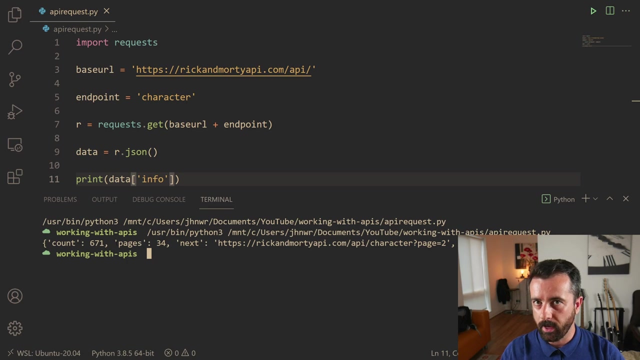 Now we can access the keys using a square brackets, like you do in a dictionary, and I'm going to type info. Let's see what we get back now. So now I've returned just the information, part of the response, And what we want to do here is we want to grab the number of pages because we want all of the responses, all of the characters. 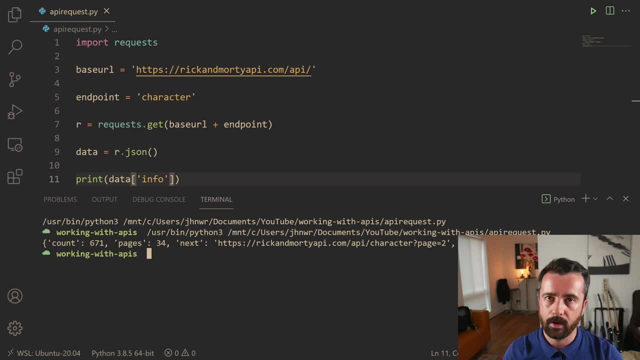 Sorry, from this API. So we're going to go ahead and we want to know how many pages there are now. You could grab the next page length when you go through every time and just do a request on that. You could absolutely do that. 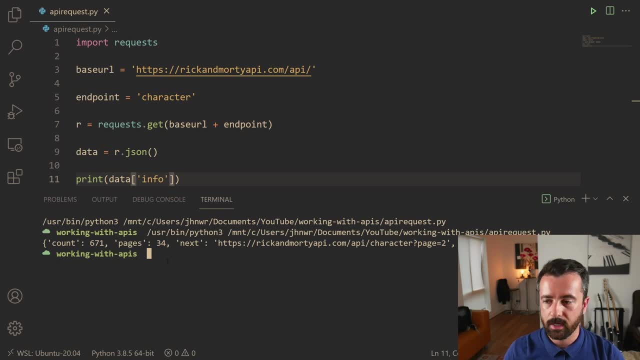 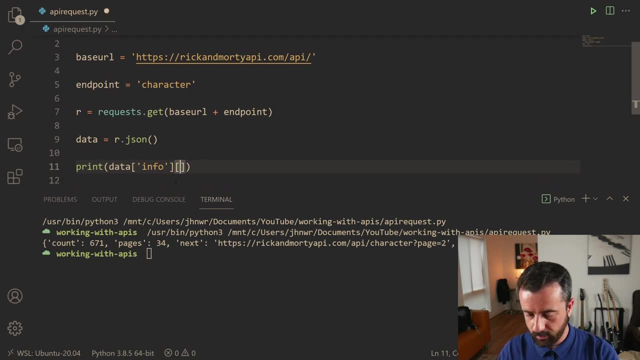 But generally I like to make one request to the start, to know what we're dealing with And then do it that way. So I'm going to say we're going to go for, let's do pages. So again we're going to reference the key of pages and this is going to return the integer of 34 there. 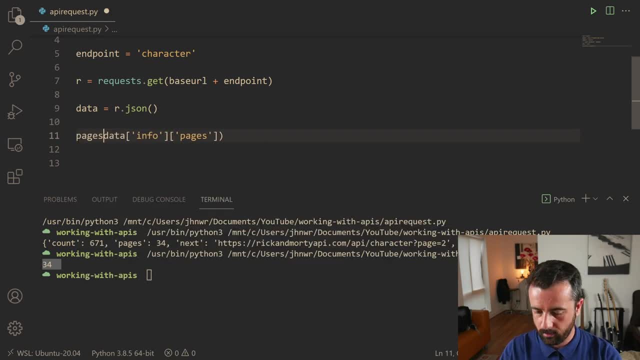 So we can save this into our variable that pages. So now what we want to do is we want to work out what parts of the other bits of information that we want. So let's go ahead and do print data. Now, if we come back to the 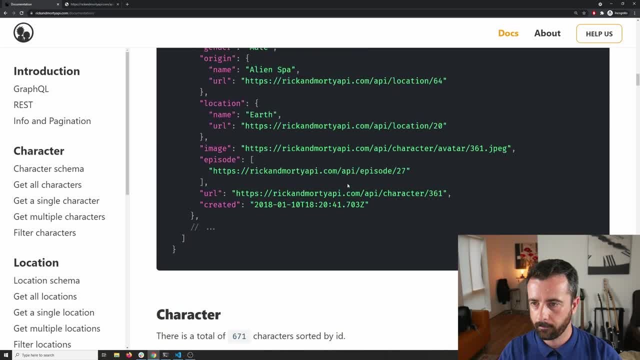 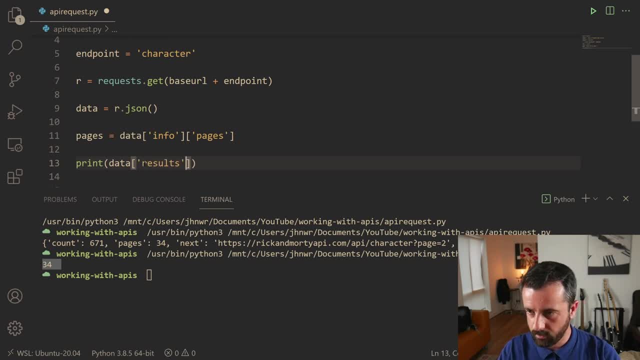 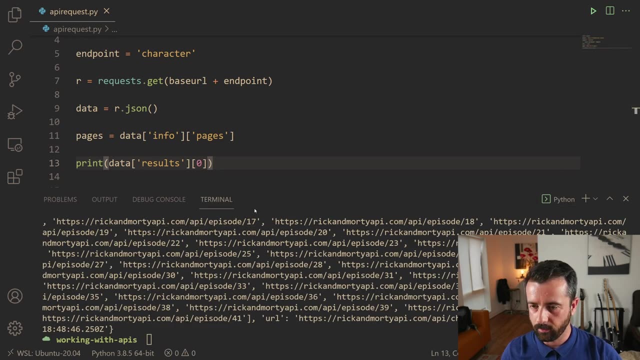 documentation. it shows us up here. We get results. Now this is a list, So I'm going to come back and I'm going to say print data results and I'm going to ask for the first item in that list. So let's run that and we can see that we get this information back here. 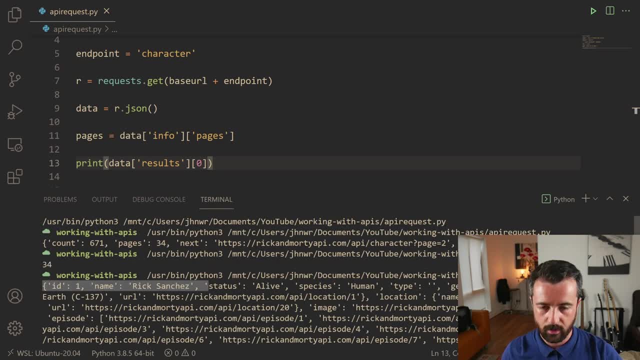 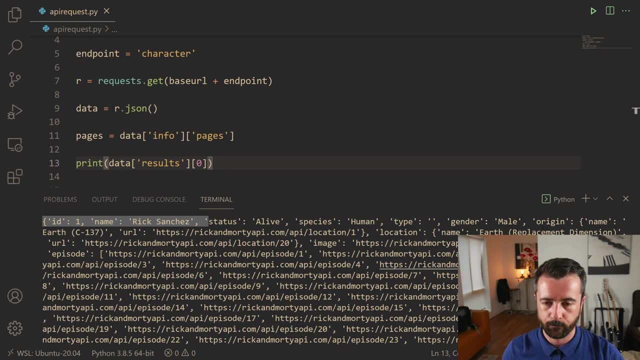 Now, within here, we have the ID and the name, et cetera, et cetera, And then some other keys that we can access, and then we can see we have all of the episode information there. So let's do, let's print out the name. 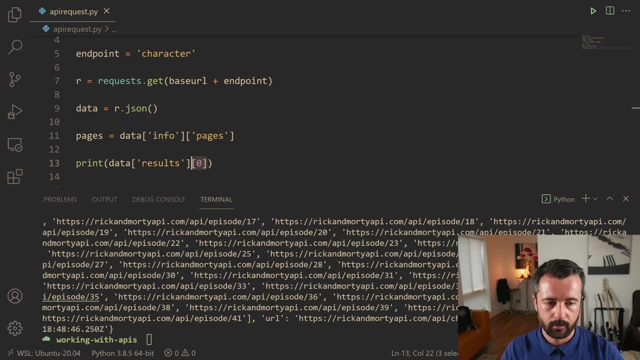 So we're going to go, we're going to stick within our first item on the list, because we're just working out what bits of information that we want And I'm going to say name, So let's print that. Okay, so we get the name and then let's save that. 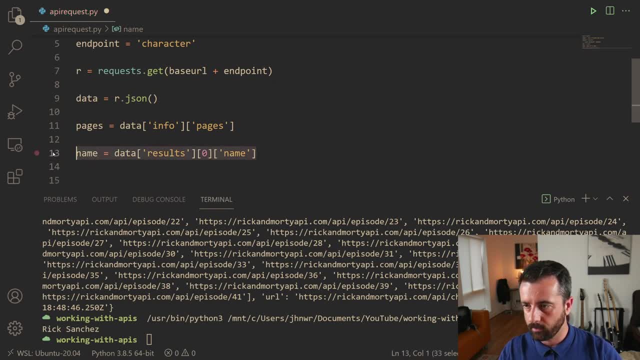 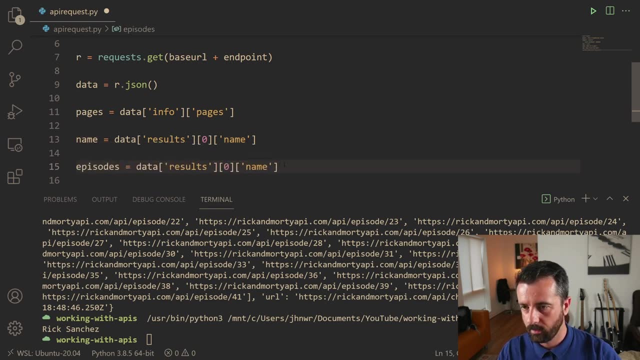 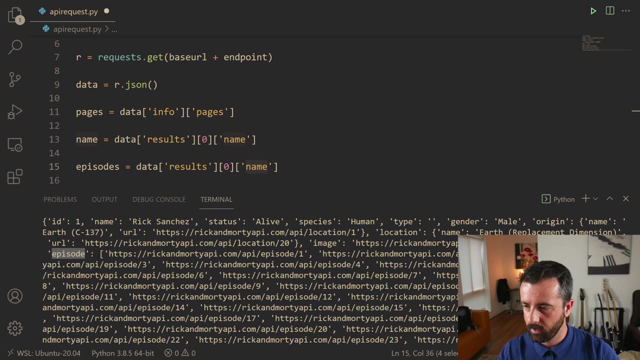 So let's do. name is equal to, and I'm going to copy that and I'm going to say episodes and we'll do. if we look for the key up here, we can see we have episode and then it returns a list, Not that episode. 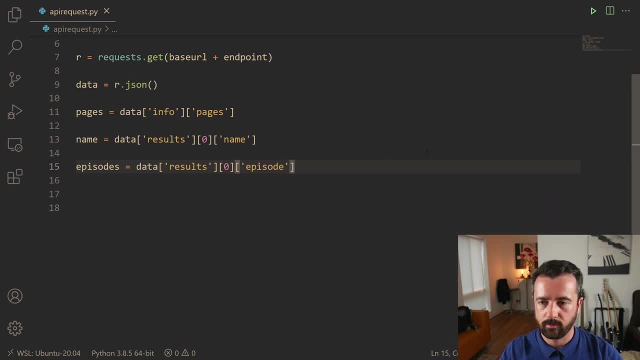 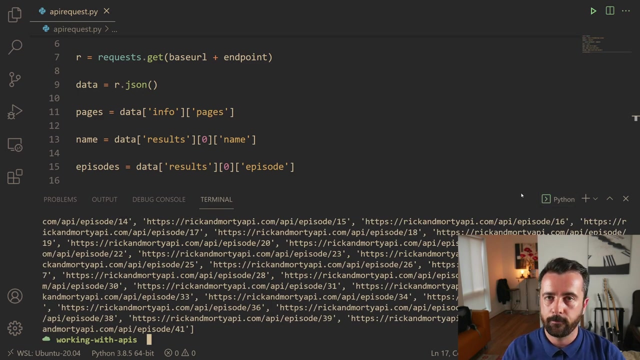 So I'm just accessing different parts of the JSON data. Let's remove that, So it's a bit clearer, and let's print out episodes. Okay, and there we go. There's our list back Now. it's worth mentioning at this point that if you're new to this and you're still trying to work out how to interrogate the 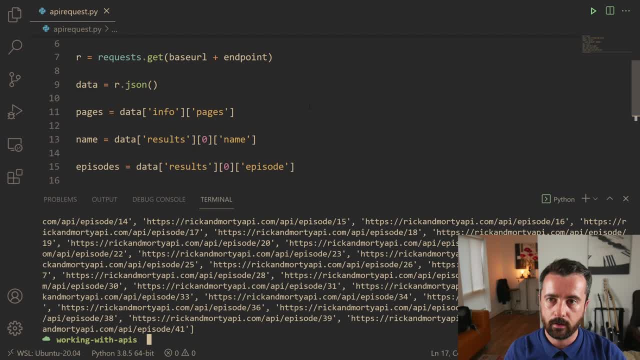 JSON data properly. don't keep sending requests to the server. Go ahead and save the response. You can just copy and paste it out into a JSON file and save it to your hard drive So you can just work out how you want to get that information out. 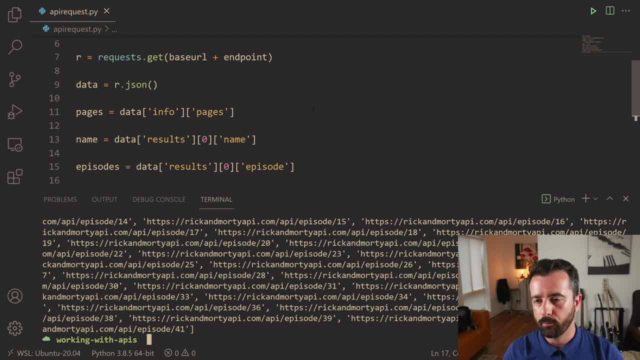 Otherwise you're just sending unnecessary requests to the server. I'm pretty confident doing it, So I mean I've only done like five or six requests at this point, So not a big deal. So what we're going to do for this is we're going to say we want to know how. 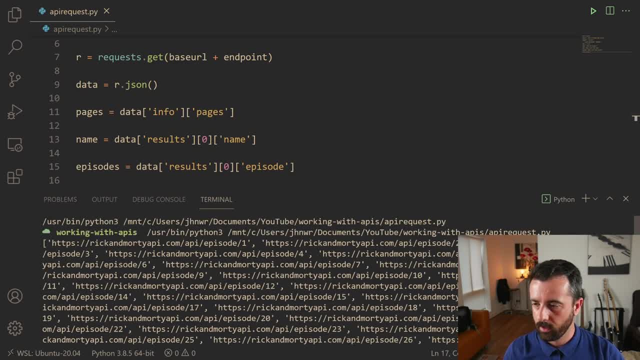 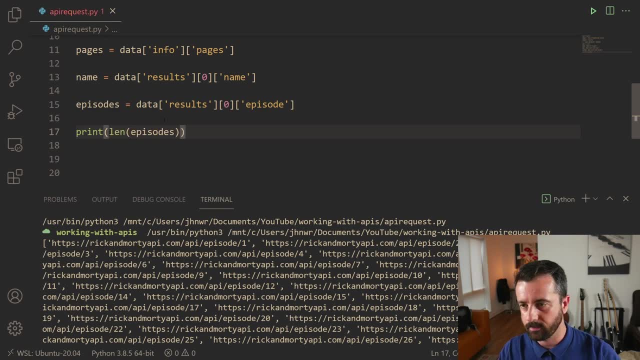 many episodes this character is in, So I'm going to do the length of episodes instead of printing out all of them. I'm going to ask for the length and that's going to give us how many there are. We can see there's 41.. 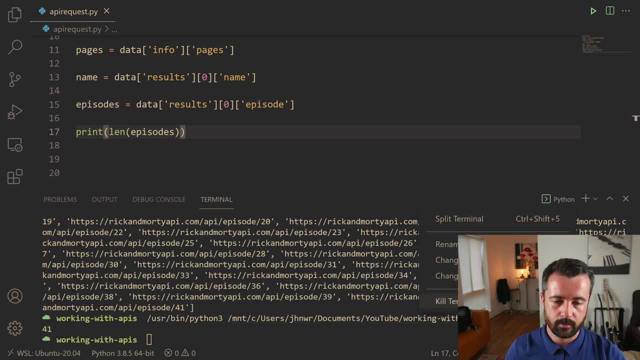 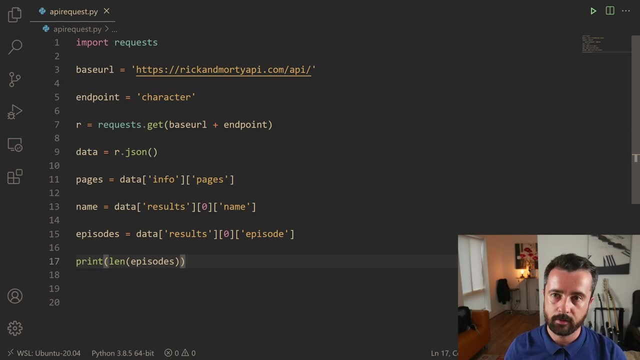 So I'm going to say that this character is in 41 episodes. So now we've worked out what bits of information that we want to get, We can go ahead and start to write our code out properly so we can make the right amount of response requests to the episode. 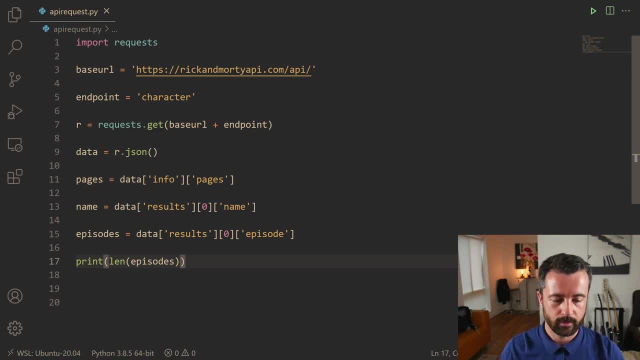 The API, get back the information that we actually want and then can then put it into a nice list, So we get total number of characters and how many episodes they've been in. Again, this is just demo information, but you'll get the idea. 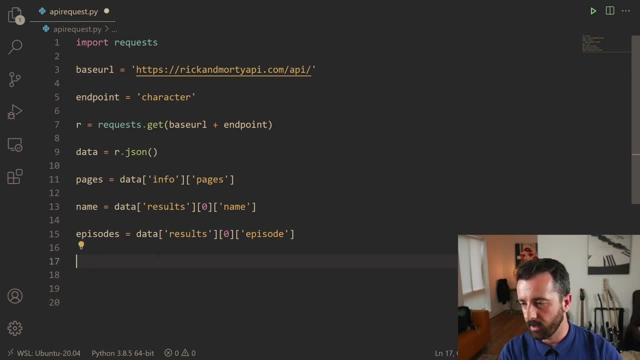 So the first thing I'm going to do is I'm going to start writing some functions and I'm going to say up here we're going to say def for defining our new function, and we're going to say main request and I'm going to say we need. 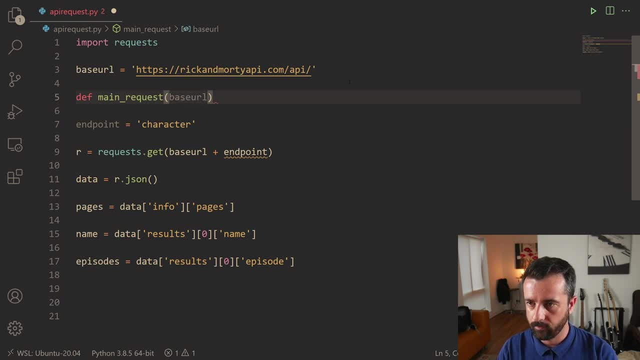 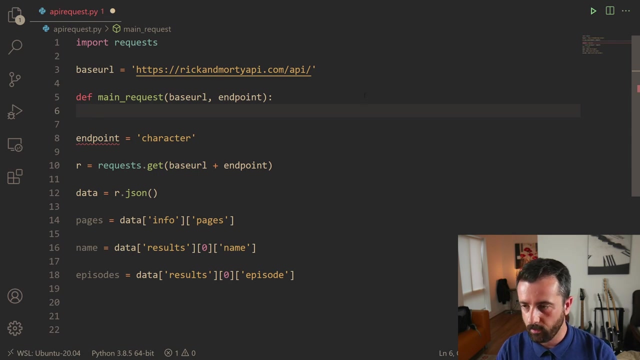 to give this a base URL And let's pass in the endpoint as well. This just means that if we wanted to, we could use this to actually go to the other endpoints of the API if we wanted to. So now we're going to put our r is equal to requestget in here, like that. 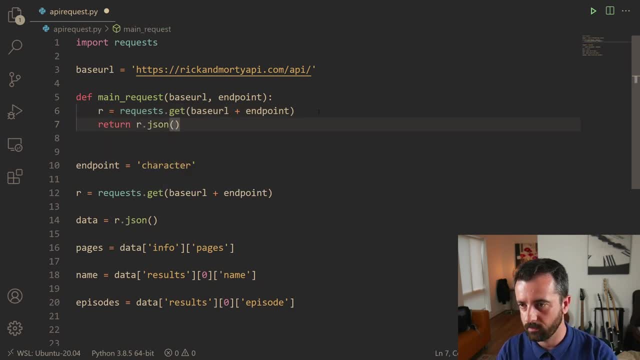 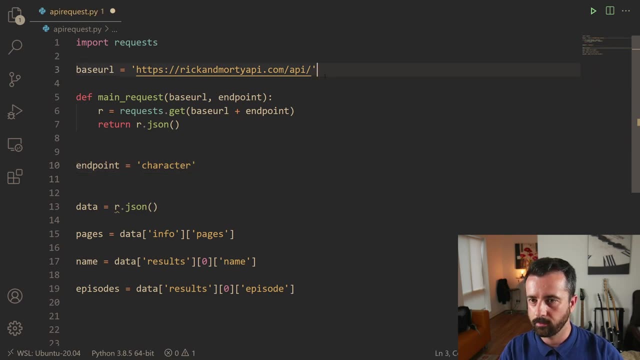 And then we're going to return the rjson, the json response here. So what we want to do now is: when you get rid of this, I'm going to move this. It's up to the top, So it's just out of the way really quick. 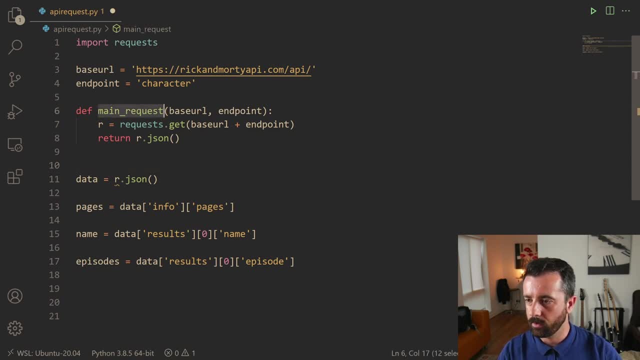 And now, instead of data is equal to this we want to do, our data is equal to main request and we are going to actually, because we've called this base URL and endpoint, Anyway, we can actually copy that out there. So now, if we run this, we should be able to get the same results back. 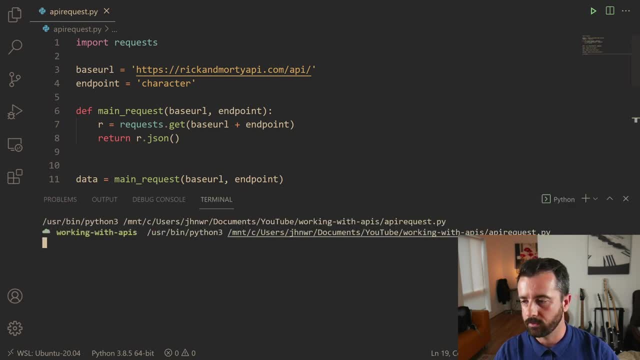 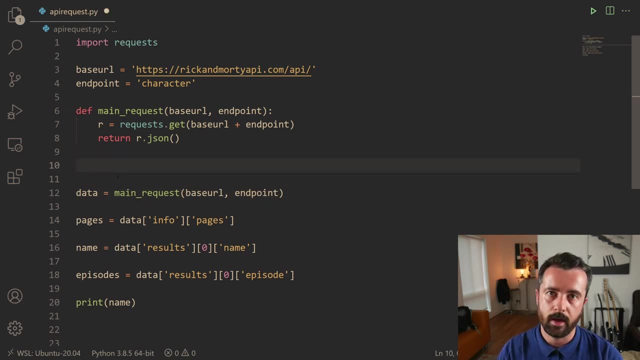 So let's just print name just to check that our function is working, which it is Okay. so now we want to, actually We work out how many pages there are that we need to loop through. So what we're going to do is we're going to say def for our new function. 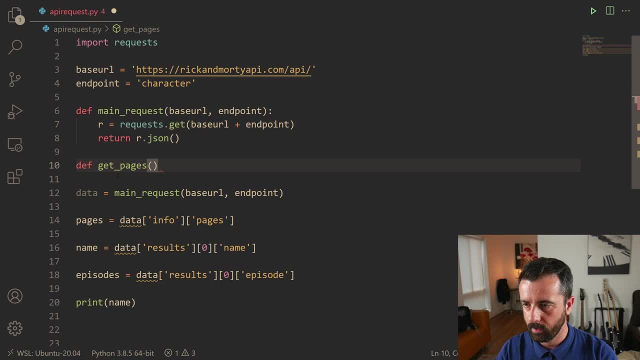 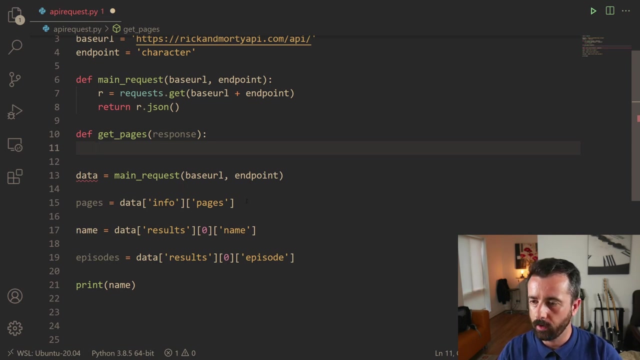 We're going to say get pages and we need to pass in the json response. So we're going to say response and now we want to work out how many pages there are. Now, as we looked here and we worked out from the info and pages we can copy, 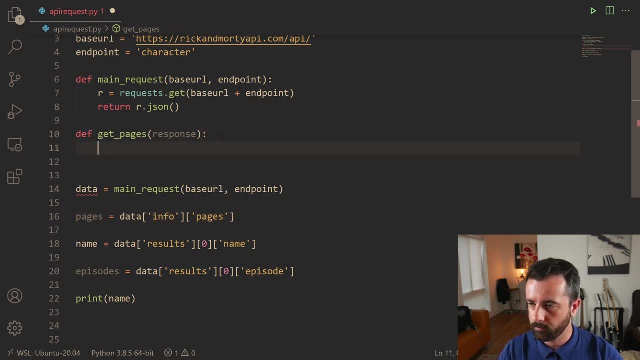 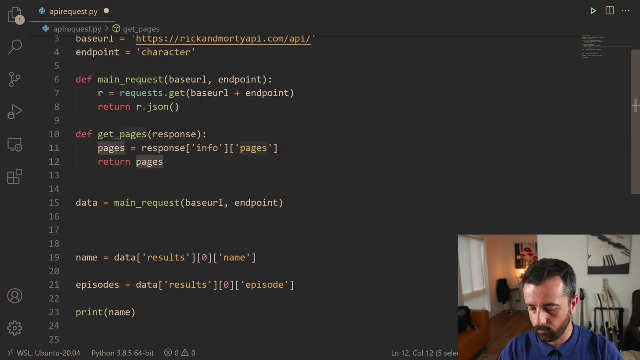 This out so we can say: pages is equal to. we just need to change this ever so slightly, because we're working with the word response and not data within our function and we can say that and then we can just return this back out. Now you can do it like that, or you can just make it easier and just put the whole thing on one line. 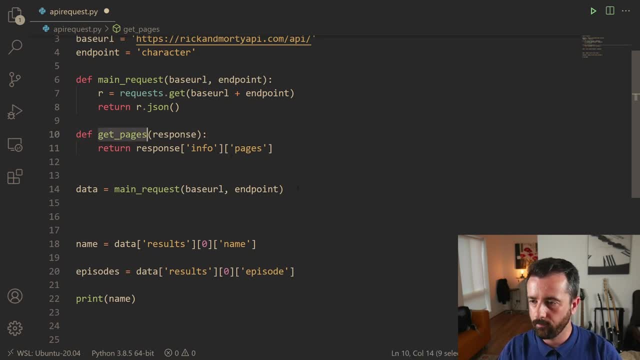 There we go. So now we, after we do our main request, if we do our, get pages on the data and we actually need to print that out And we'll remove this print statement from down here and run this. We should see 34.. 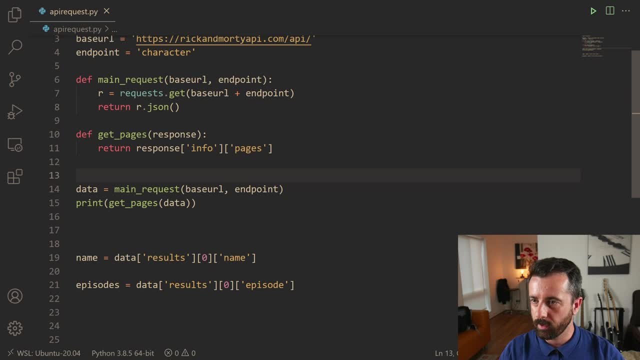 There we go. So now we can say that we're making a request and we can work out how many pages we need, And so what we're going to do now is we're going to write a function to actually work through the character information on each request that we give it. 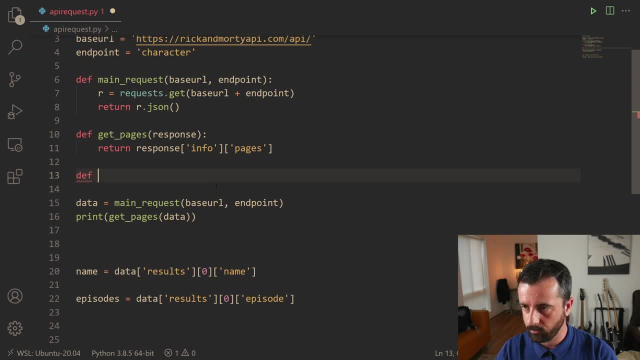 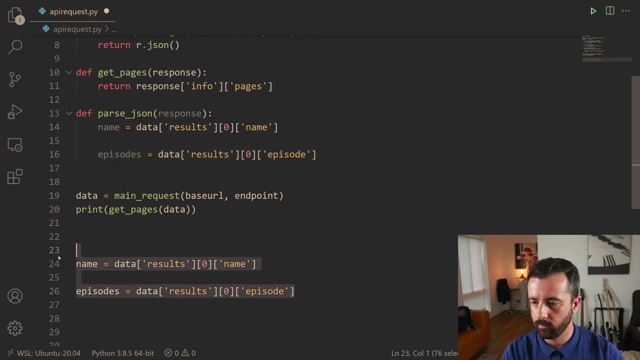 So let's say def for function and we'll call this one past json and we're going to give it the response Again. So now we want to put these two in here. This is where we found the information, So I'm going to remove them from down here. 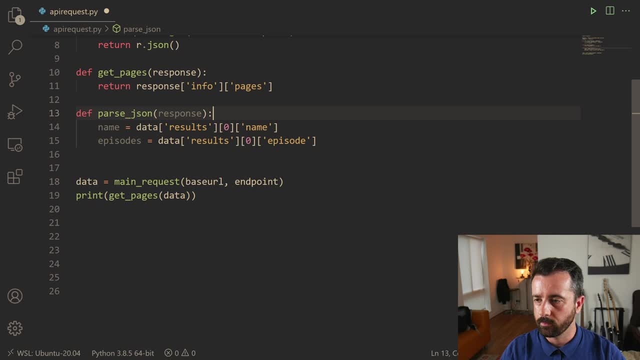 But what we need to do is we need to make this into a loop. So, instead of it like this, because here we're actually indexing the first item in the list, So what we're going to say is for item in response, and we want to access the results key, which is we've got here. 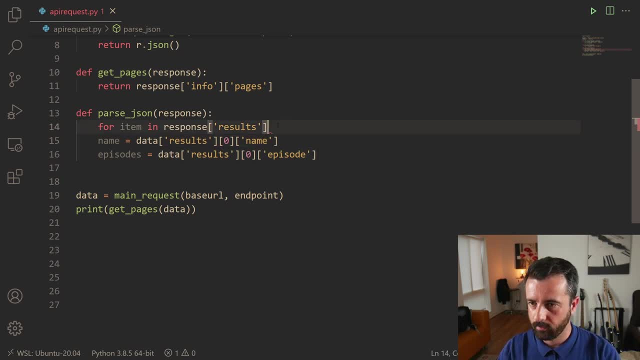 So we can remove this, This part. we want to say print item and we need to reference the name and then the episode, But we want item. Sorry, we want length because we wanted to know how long that list was of episode. there I've got too many things going on. 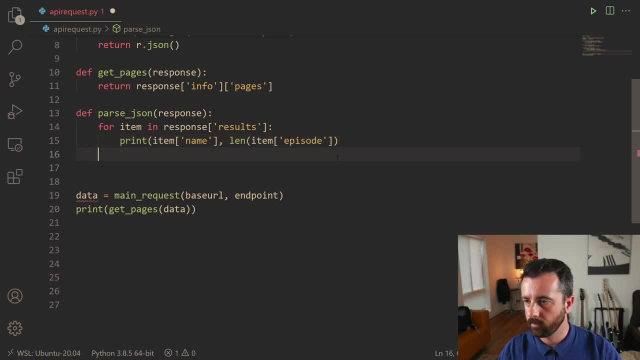 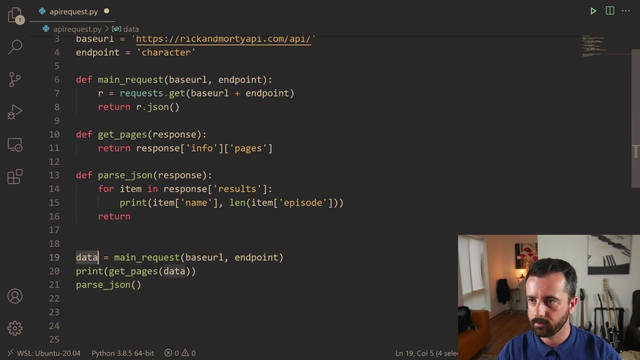 There we go, So I can get rid of these now. for the moment, I'm just going to return this Function, So I don't get any errors and I'm missing a bracket, So let's put that in. So now we can do our past Jason function and we can say we need to give it the response, which in this case is data, because 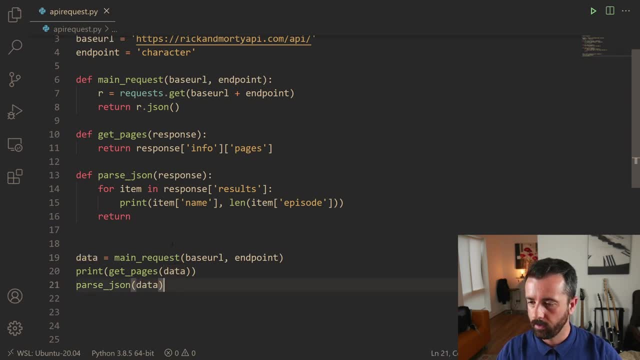 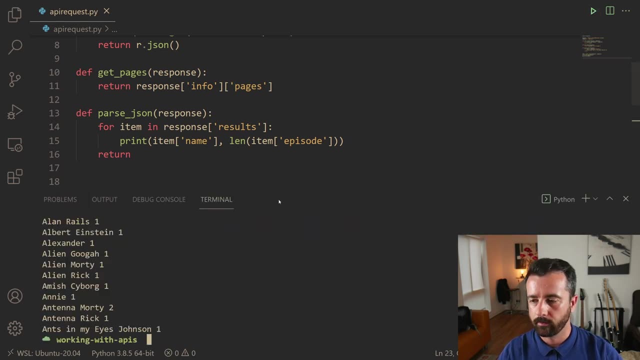 the response is coming from the main request function And we have put in a print statement in here temporarily just to check that it works. If it doesn't, we can tidy up our errors before we crack on. Right, There we go. So it looks like we've got our 34, which we are printing out from our get pages. 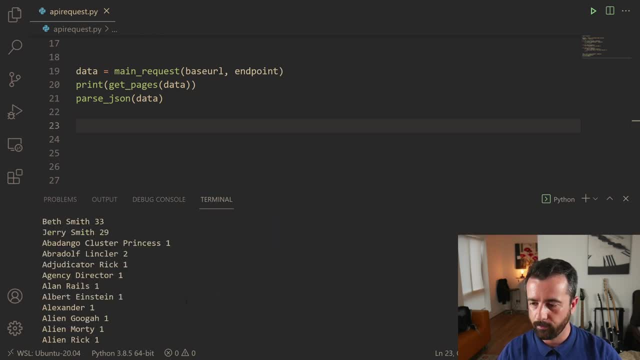 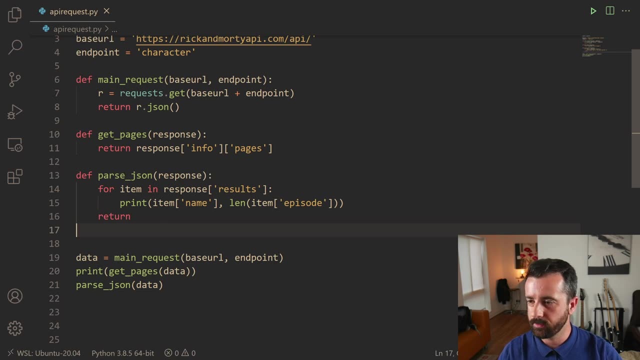 And we have List of characters and the number of episodes that they've been in here. So we're halfway there. So let's get rid of that. So now what we want to do is we want to save this past Jason part into a dictionary so we can actually do something with the data. 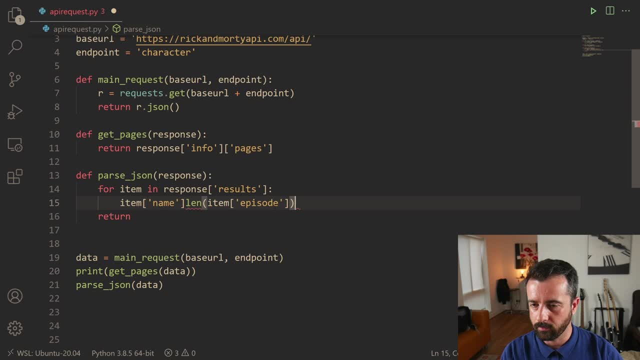 So, instead of printing these two things out, I'm going to put them on separate lines, just like this, And we're going to say our character, or we'll just call it char for now, and we're going to create a dictionary that includes These two items. 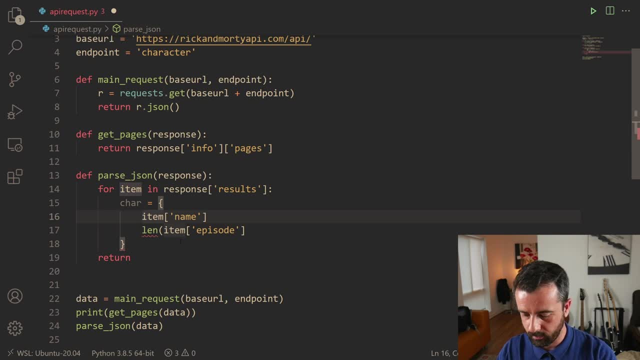 I'm just going to indent that in there and we're going to say the key is name and that is equal to the item name, And then the number of ep- oh I need, there we go- is equal to that there and we're missing our bracket there. 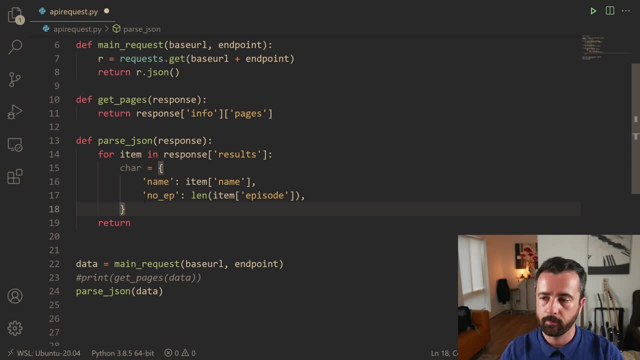 We have our character dictionary here that's populated by these fields, but we need to add them all to a list so we can actually return the whole list From this function. So just at the top here, I'm just going to call this character list and we're going to copy that. 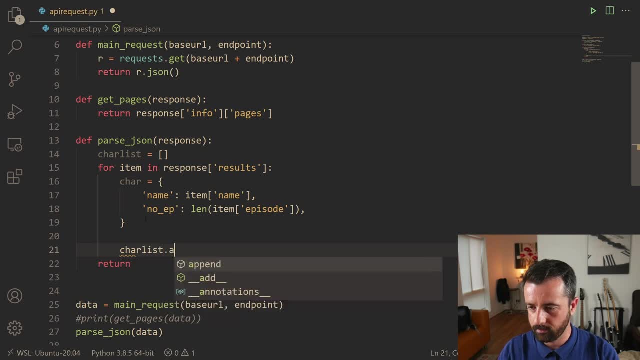 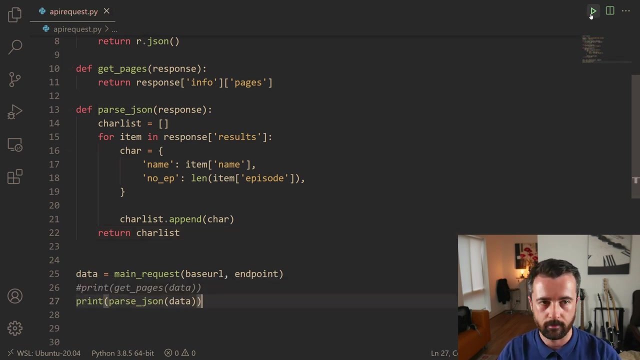 And here we're going to do character list: dot, append The character that we are adding and then I'm going to return out of the whole function, the character list. So now, if I print out what comes out from this function, just to see if it's right- hopefully it is. 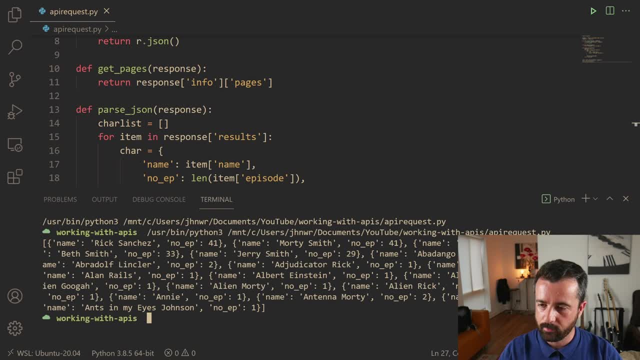 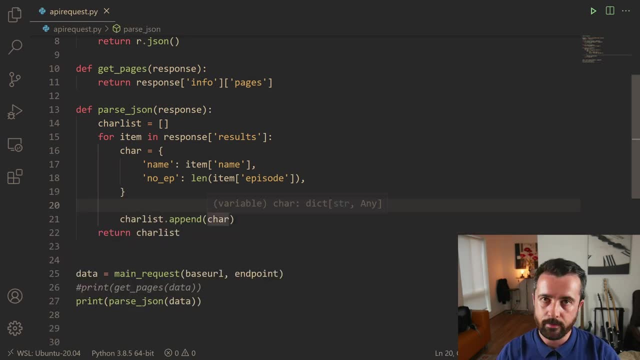 There we go. So now we have a list of names And the number of episodes that they've been in, just like we had before, But it's in a bit more of a useful format now. Now we've got that working. We want to work with the pagination, which is why we have this: get pages function. 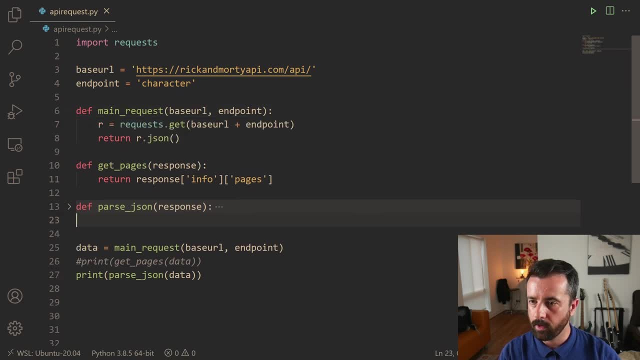 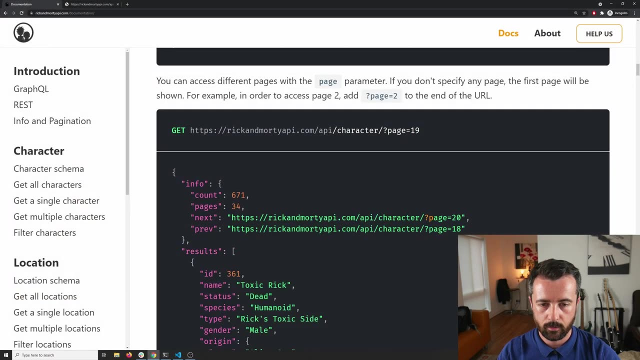 So let's collapse these ones out of the way. So we know that our main request works here, But if we look at the documentation again, we can see that it has this question mark and then page is equal to 20 at the end. 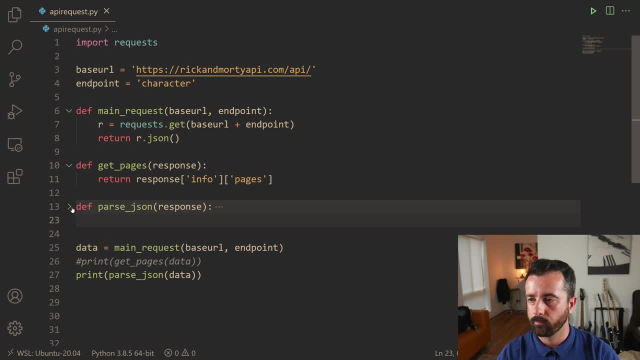 So I'm just going to copy that. What that will do is that will work. Tell the request which page to work with. So I'm going to add that in at the top here. So I'm going to say that we need to give this a number, which I'm going to make as x and we're going to do plus, and then page is equal to x, like this: 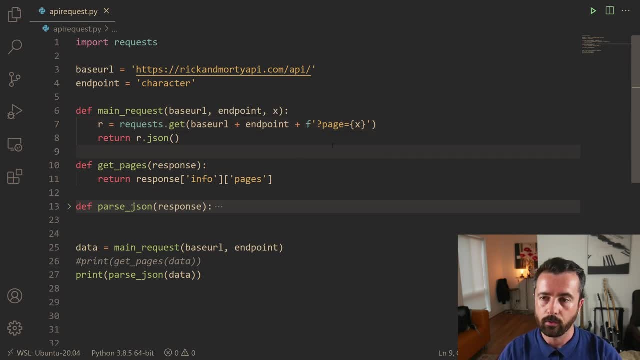 I'm going to make this an f string so we can actually add that all together. So when we make our main request now, we're going to start with a number one And let's check that That works. We get the same information back. 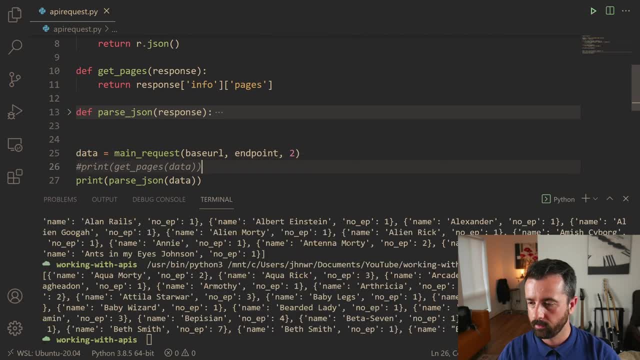 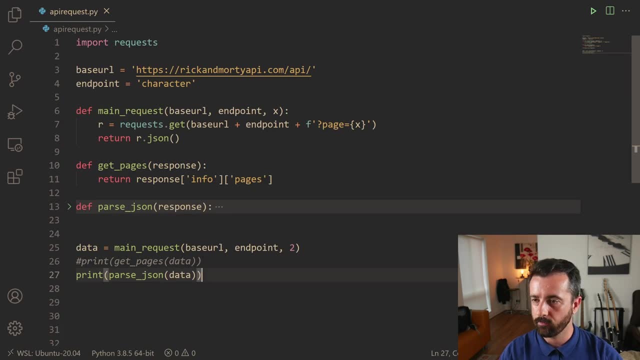 So now if we go to number two, we can see we've got some different information, which means our pagination is working. So we can just use this main request function- So once we do the first one on page one to get how many pages there are and pass that part of the data. 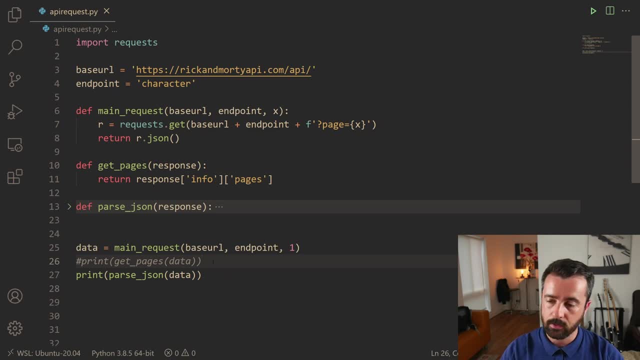 What we can do is we can say 4x in range. So let's get rid of this. Oh, not get pages, Let's just get rid of the print part so we can say 4x in range And we can pass in our get pages. data function there. 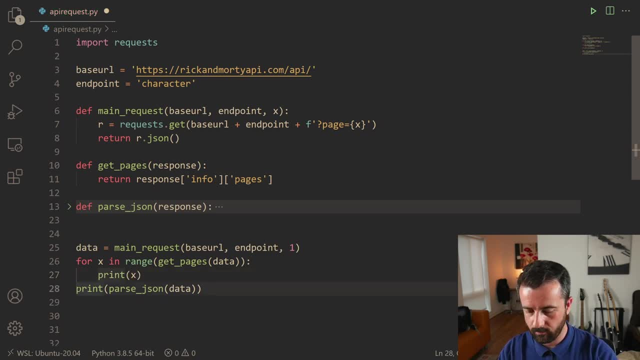 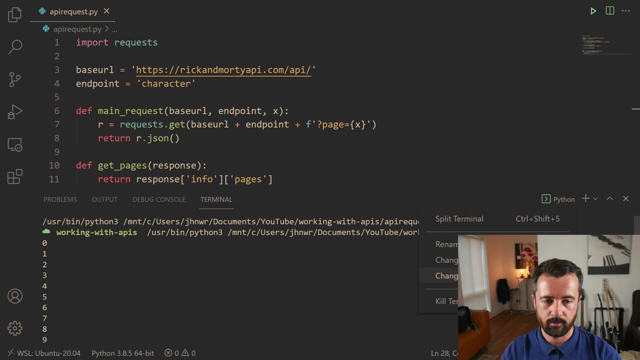 We can print x. So if I just get rid of this for the moment, as we can see it goes to 33 and we actually have 34 pages and it starts at zero. We just need to shift that over. So I'm going to say 4x in range. 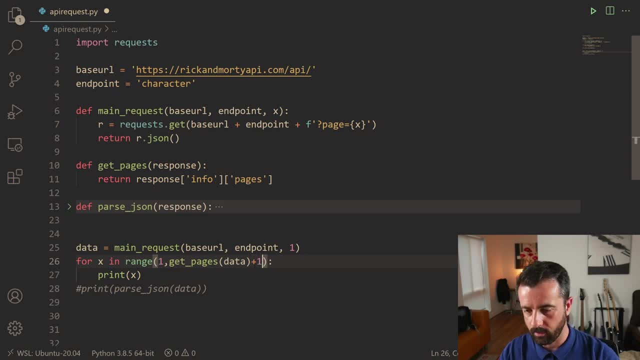 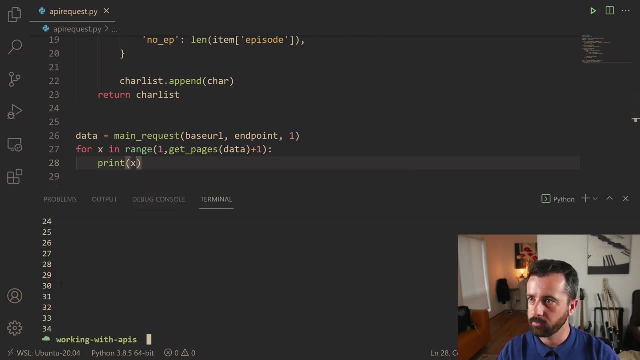 We're going to start at one to get pages data plus one. So if we now print x, we should get one to 34, as opposed to what we had before: Zero to 33.. There we go: 34,, one to 34.. 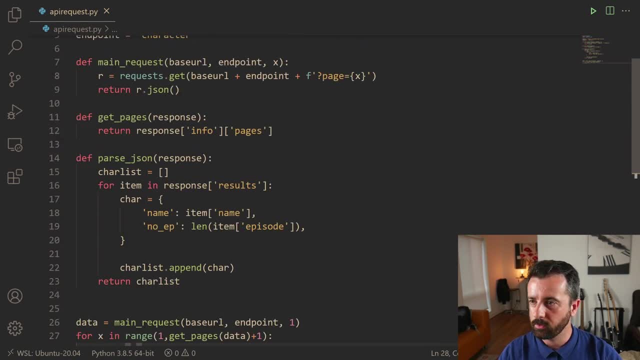 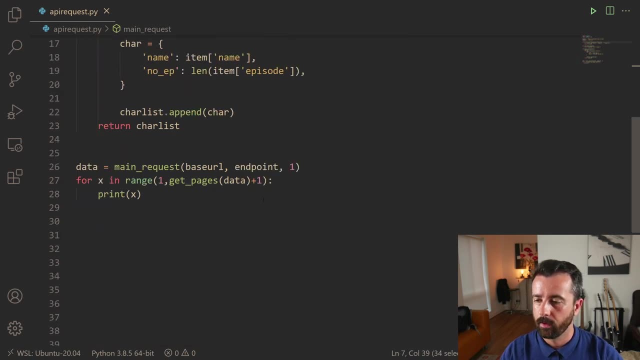 So those are going to be our page numbers. So what we want to do now is we want to use our main request function, which basically, is the one that returns the json data. I'm going to copy that out. We're going to put this in here. 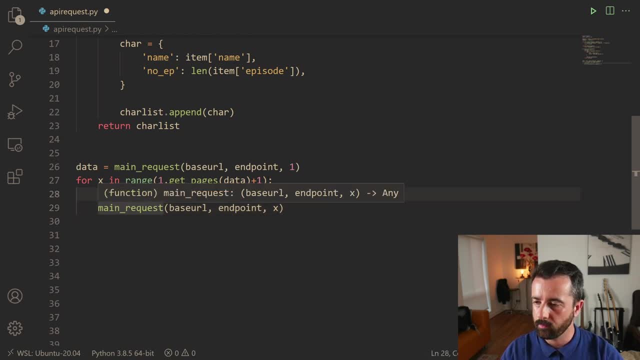 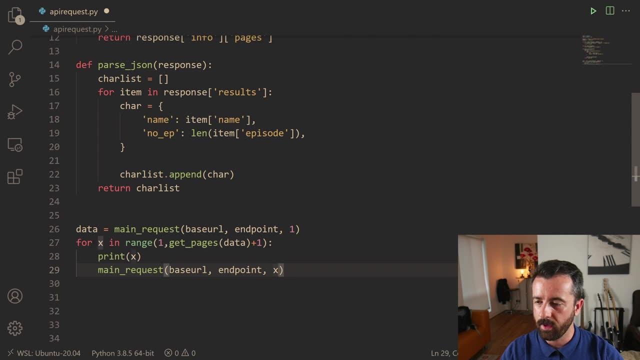 Now we leave the print statement in so we can see the pages go by, but we're going to do main request of the base URL and the endpoint, which is: are both up here, which is correct, And then x, which is for the x or the page number. 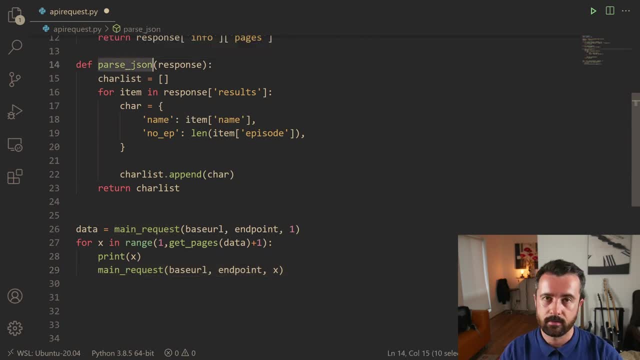 So we could store this into a variable, but we actually want to pass the information from this. So I'm going to grab our past json function and bung that in main and we're going to put that there. Now what we want to do is we want to actually store all this information that comes out and we get a list out of this. 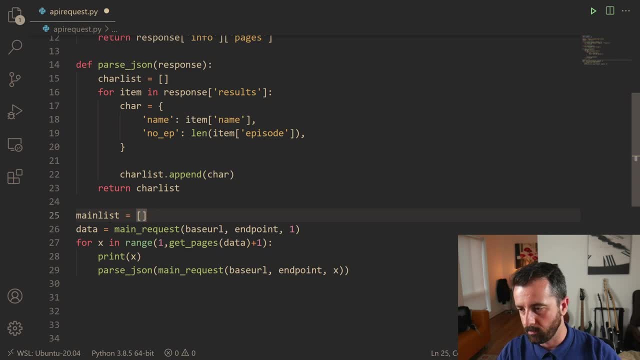 We can actually have a new main list, Probably not the greatest name, and we can put that in here. But what we can do is we can do dot extend. So this is basically going to add everything that comes out of that list into this new list as we go through each time. 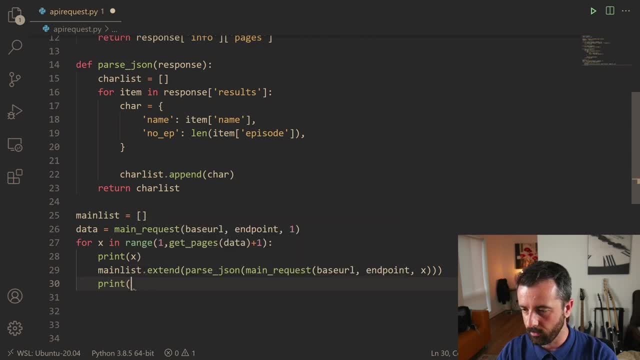 So now if I do print the not inside my for loop has come out of my for loop and we do print. let's do the length of the main list. This is a good way to find out if you have sort of the right amount of records. 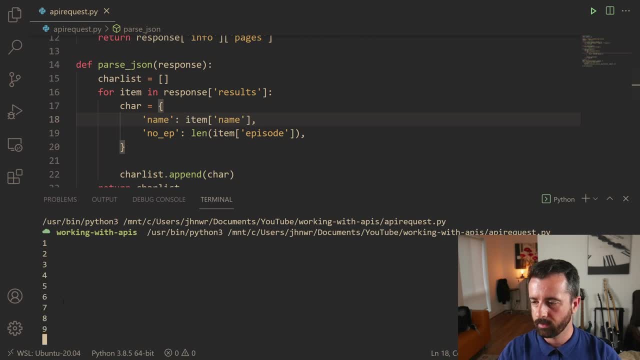 I think it was 607.. One we were looking for. So we can see this is the request we're making here to the server. We need that to go up to 34 pages, hopefully 671.. So we've got the right amount of results. 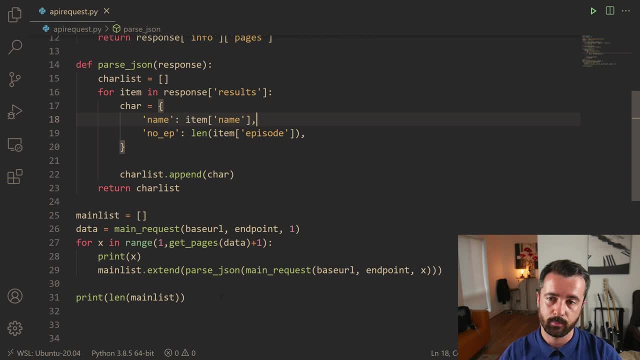 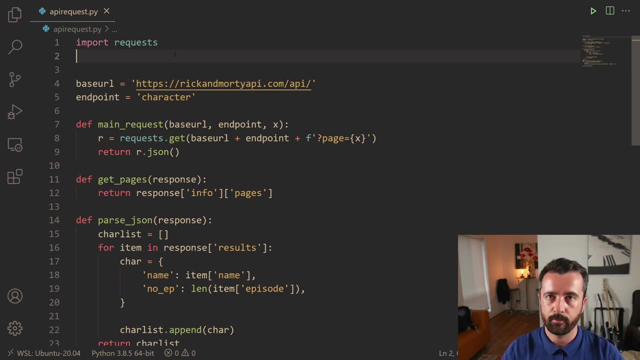 So I'm happy that now what we can do is we can export this to a csv file. So let's import in pandas Now. pandas is basically a really powerful data science program and to use it for just creating a data frame in a csv file. 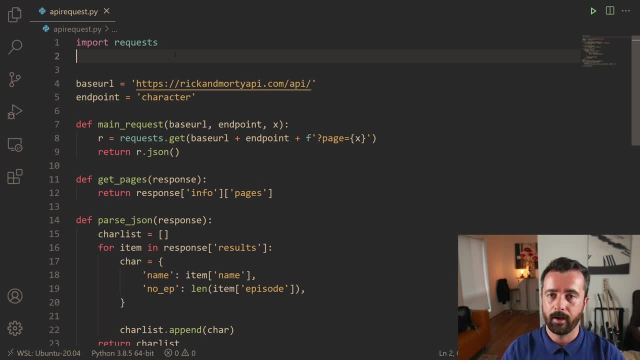 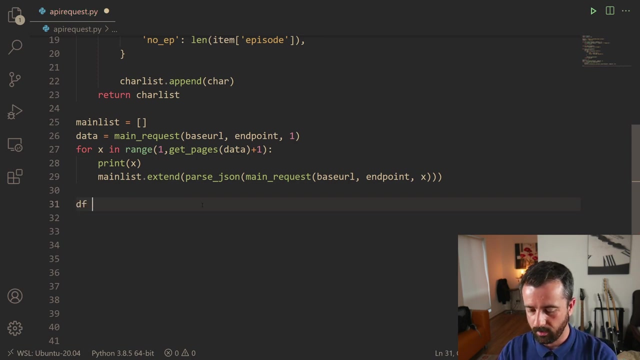 Possibly overkill. However, it works really well and I don't know. I'm happy with it. So I'm going to import pandas as pd again. pip, install pandas if you need to. now, instead of printing the length of the main list, What I'm going to do is I'm going to say df for data frame. 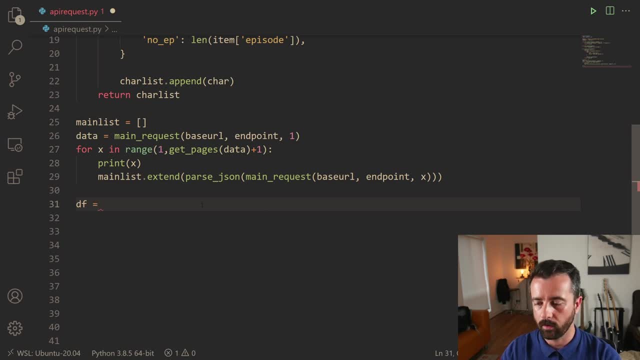 Make sure you call your data frame- something useful when you're actually writing your code in an actual project, Don't just write df, because it'll be confusing- is equal to pd dot data frame- Main list. So then I'm going to print df dot head and then df dot tail, just to double check that the top and the bottom of our data is different. 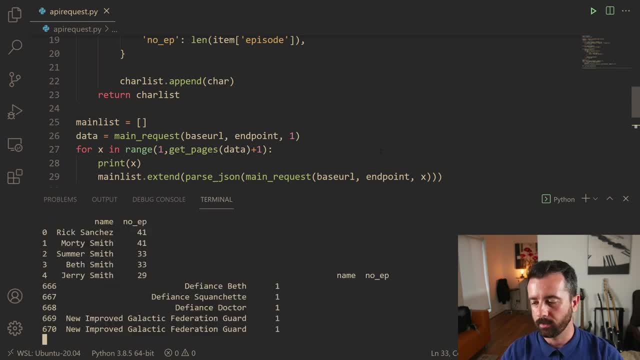 And we haven't like duplicated it up or something like that, and then we can see we can work on exporting it. So I have actually got here. 670 will be 671.. This looks like a duplicate If we go back to our actual response, and this is page 30.. 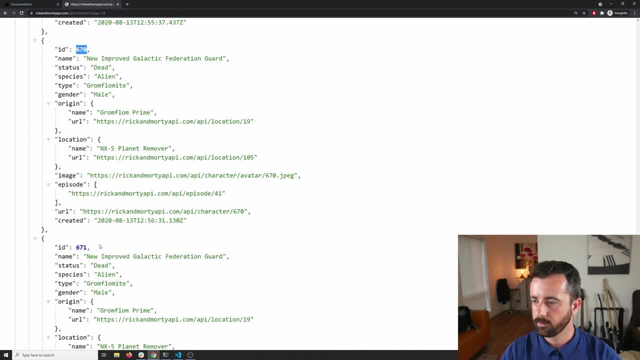 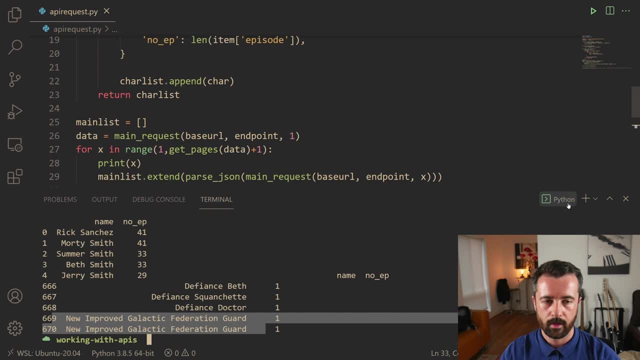 For we can see that we do have two lots of the new improved galactic federation guard And, to be honest, we should probably stick the ID in there as well. That would make a lot more sense. So I'm actually going to do that. 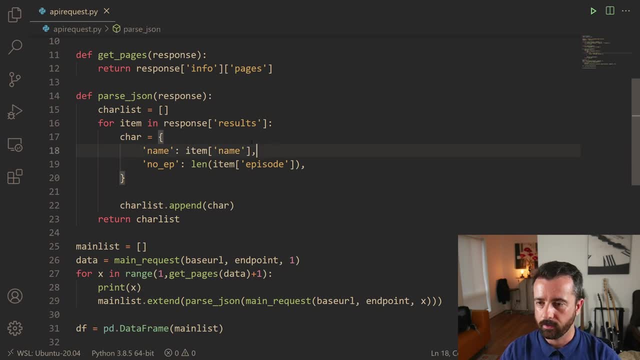 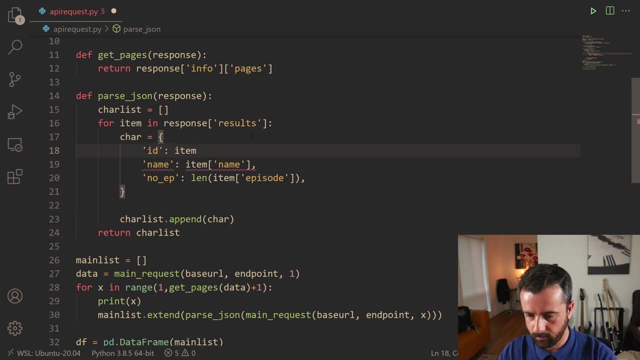 So what we're going to do is up here in our past, Jason, we can actually put the ID in. So I'm going to make a new line in our dictionary and say I ID is equal to item ID, because the key was the ID key. 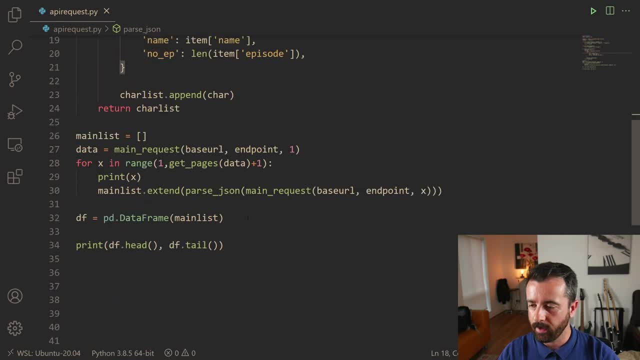 We can see it there. So now I've added- added that in instead of printing this out. I'm going to do df dot two csv. This is why I use pandas, It's so easy to do this, and we're going to call this character list dot csv. 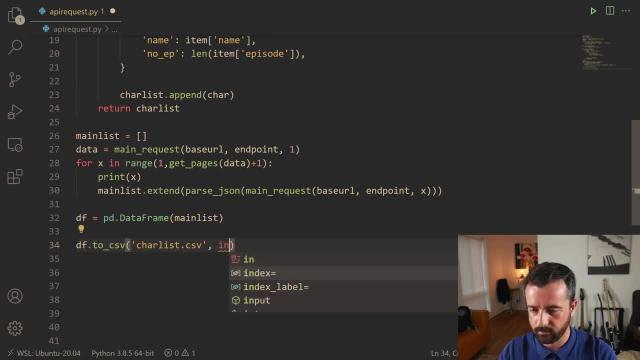 And when working with pandas in this lot that I always tend to do, index is equal to false, because generally I don't want the pandas index, which is the zero index down the side. I just want it to look like you would expect it to. 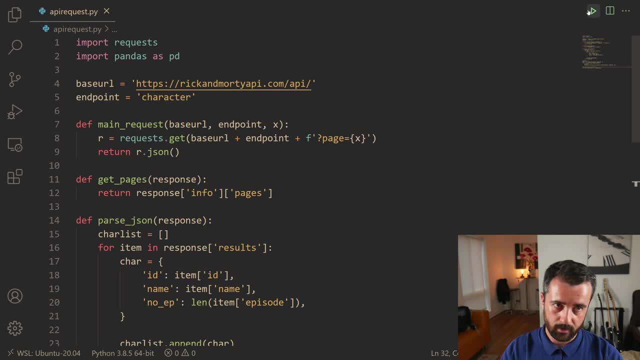 So now I'm going to save that And I'm going to run this again and this will be the last request I make to your API, I promise, and we will have back our csv file of the all the characters that have ever appeared in this show and how many times they've appeared in each one with the episode. 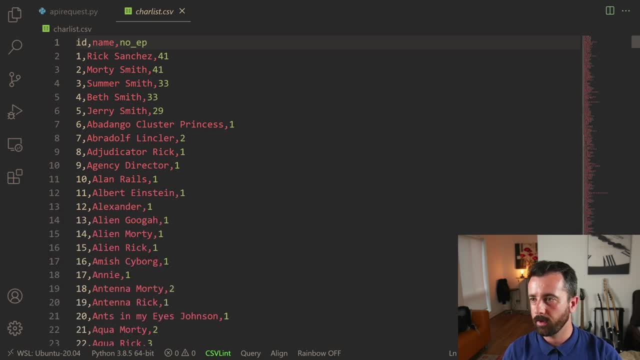 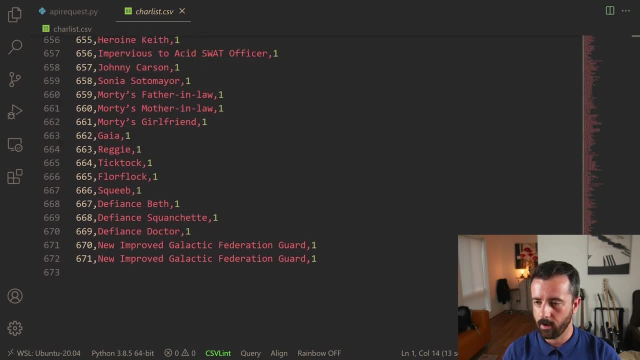 So let's click on that, Let's close this so we can see- and now we have our ID, our name and the number of episodes, all the way through down to all these characters who only appeared once, including our new improved Galactic Federation guards, Who are the newest characters, if the ID number is anything to go by, which I'm sure it is. 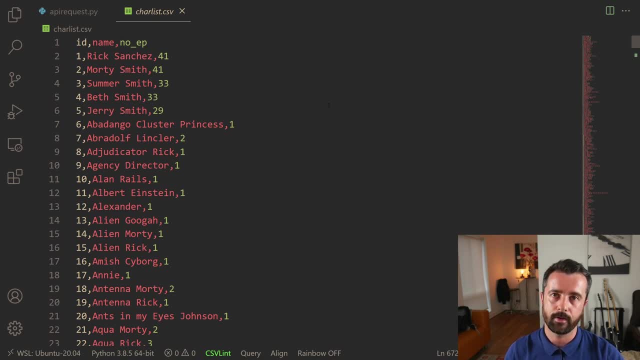 So that's going to do it for this video. guys, Hopefully you've got a good understanding now of how you can start to work with an API in python and you can make your own queries. There's a lot more to it than this We could actually filter, but I'm not going to cover it. cover that in this, in this episode.